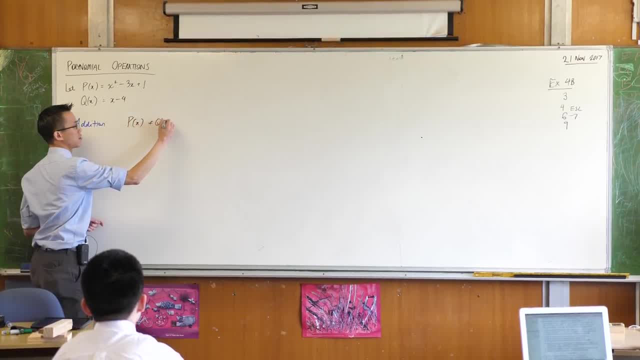 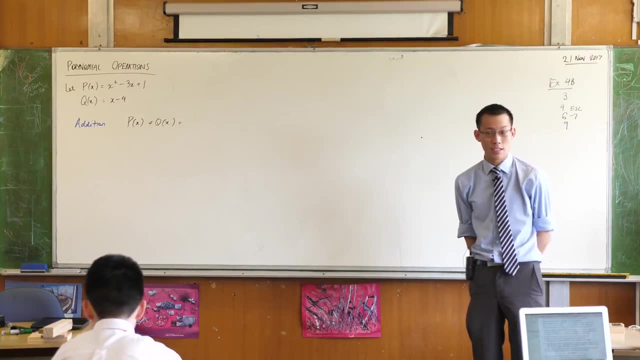 Well, if you say p of x plus q of x, then we can simply go term by term, we can collect like terms because, as you notice, there's a couple here that I can deal with and you get a new polynomial at the other end. 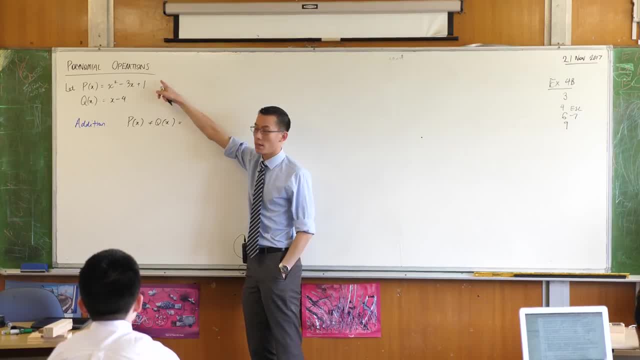 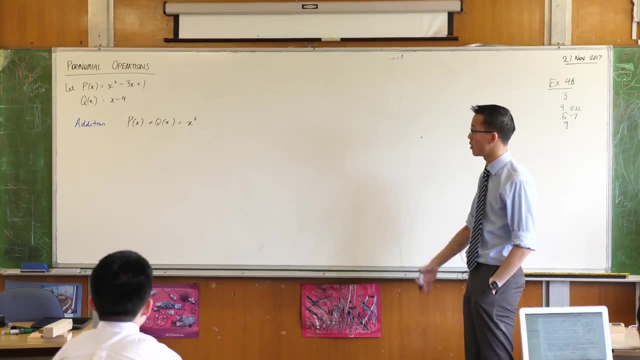 So, for example, you can see that there are only x squared terms in p, right? So I'm just going to write the x squared term there. There are x terms in both p and q, so when you collect like terms, what do you get? 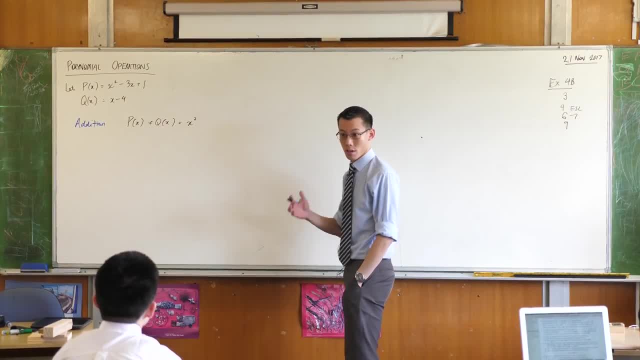 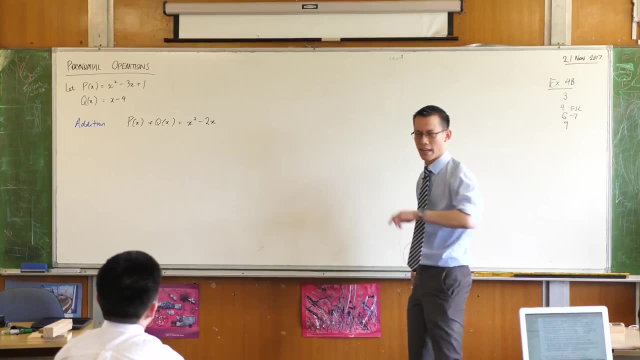 Minus minus 2x. good. And then, when you look at the constant terms- plus 1,, minus 4, looks like we're going to end up with minus 3.. Okay, so I've added these two polynomials, no big dramas. 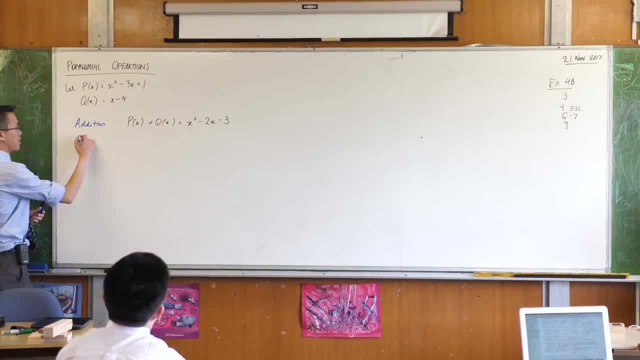 Just like adding, I can do subtraction because these are inverse operations. So instead of doing one plus the other, I'm going to do one. take away No big dramas here. So again I'm going to look at. this time order matters. 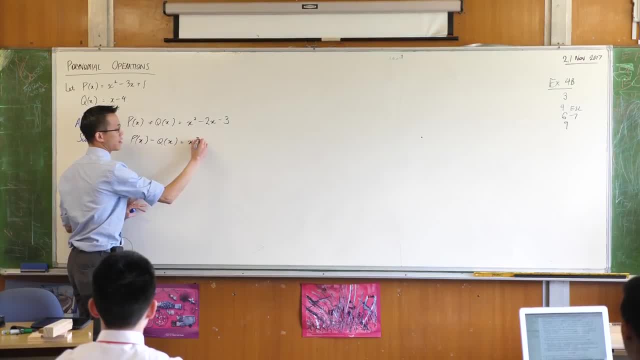 so I'm going to have to do the top one, take away the bottom one. x squared, it doesn't get subtracted. there are no other collecting like terms that happen Here. minus 3x, minus x- how many x's do I end up with? 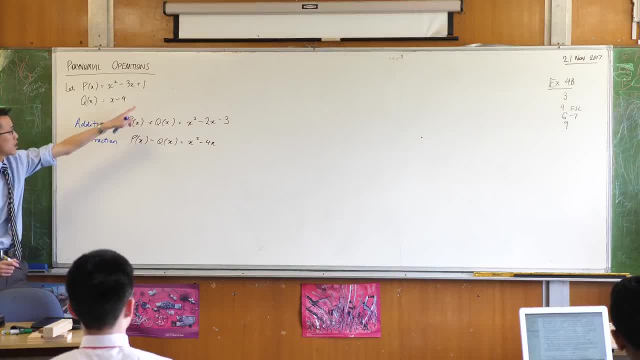 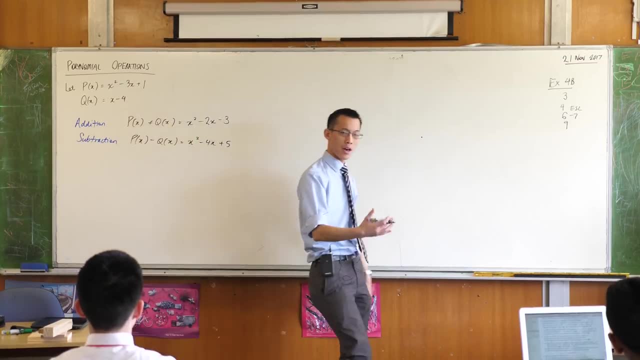 Minus 4.. And then, when I have a look at the constant term, it's 1, take away negative 4, which leaves me with plus 5.. Okay, Before we move on to the other option, I want you to notice some things about the degrees here. 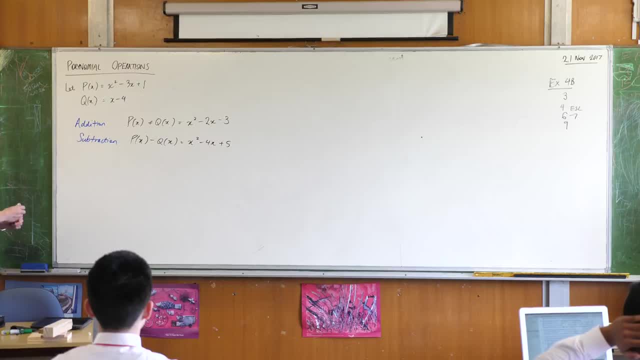 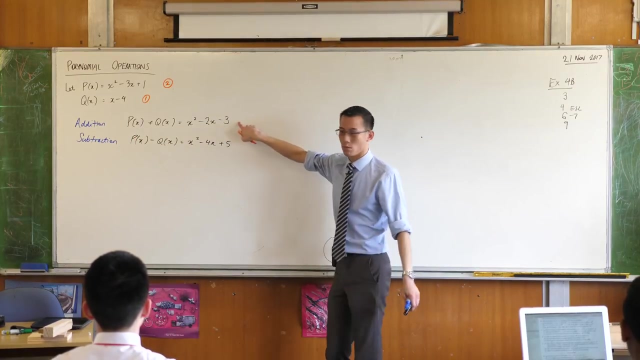 Polynomials p and q. you can tell me what their degrees are pretty quickly. The degree of p is 2.. The degree of q is 1.. And now I want you to look at the degrees of the sums and differences. p plus q: what's its degree? 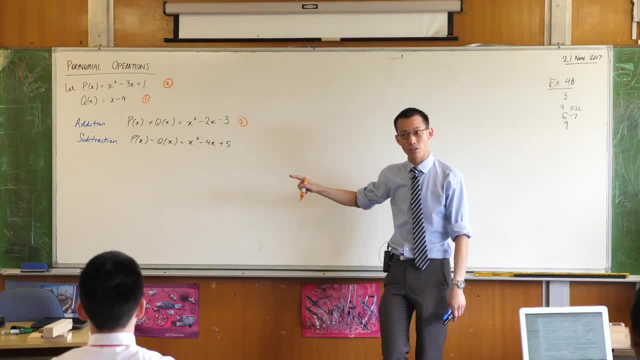 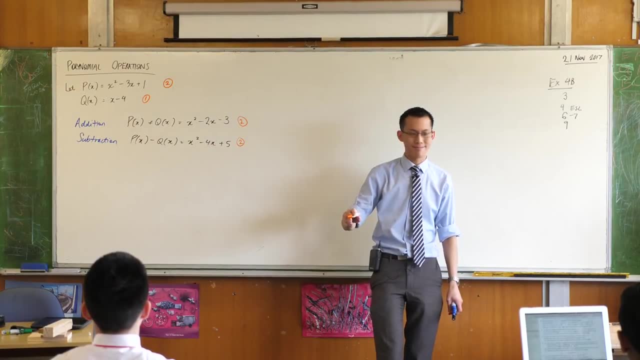 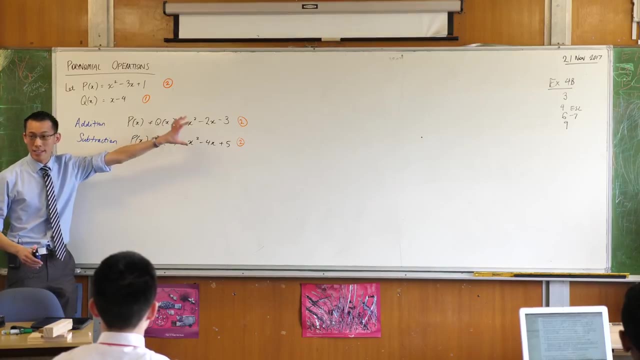 2. And p minus q, its degree also 2.. So when you add- That was just I was bordering on evacuation length there anyway- When you add polynomials you can see you end up with the degree. 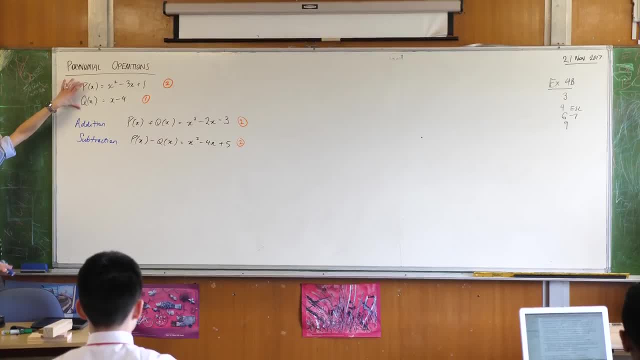 that was highest out of your original functions. Does that make sense? Or polynomials, I should say okay, So no big deal, But it starts to get a little more complicated when we look at more interesting operations. So if I instead don't add or subtract, but multiply these two, 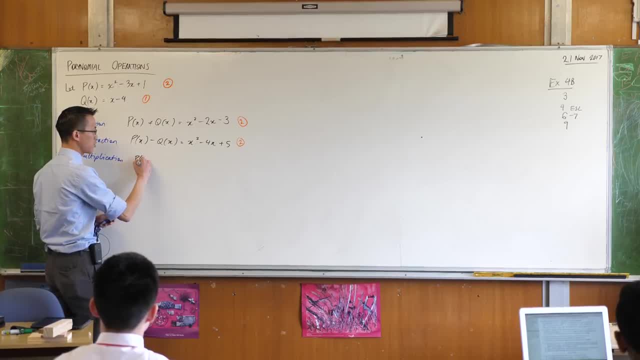 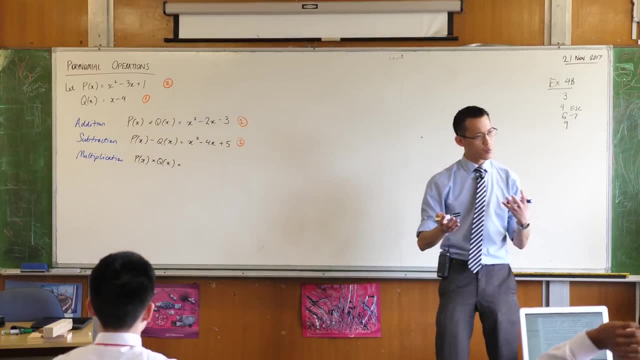 if I say p of x times q of x, I want you to make a prediction. What's going to happen to the degree? Well, you've got degree 2 times degree 1.. And these are just some. Well, you're just going to do some index law stuff, right? 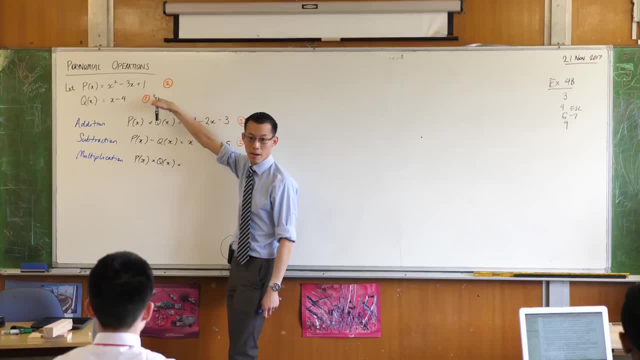 So when you've got stuff which has a power of 2 and you multiply it by stuff which has a power of 1, what do you end up with? You get a power of 3.. So the degree that I'm going to get here, 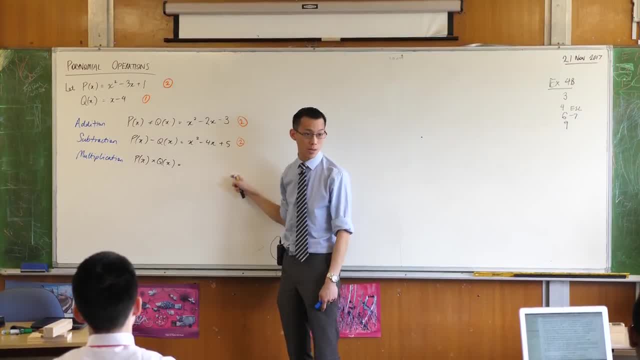 if you put together a quadratic and a linear function, you'll end up with a cubic of some kind And we could work out what this is. It wouldn't take. It wouldn't take too long. I'm going to multiply everything by x. 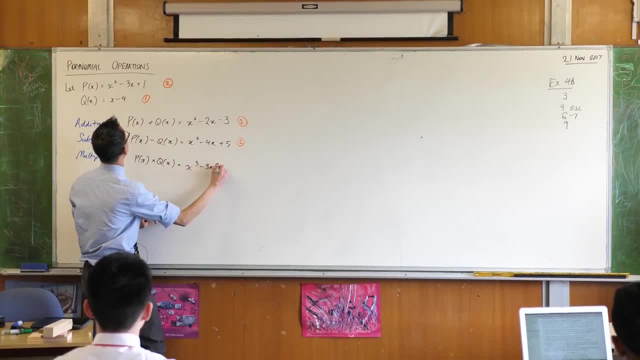 That gives me this Like so, And then I'm going to multiply everything by negative 4.. So that gives me: Let's see here: Oh, that's a plus. Did that look right? Did I expand? Get rid of my brackets okay? 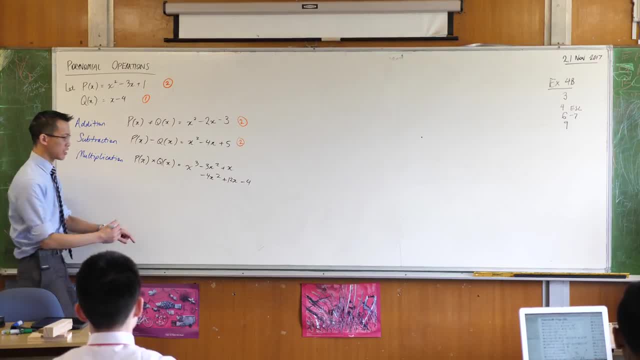 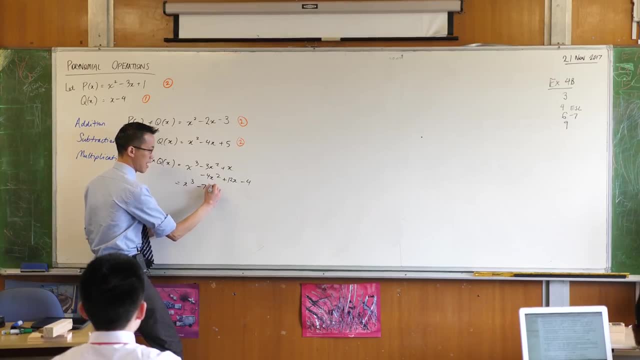 You can see why I've written it in two lines like this. Can you see why? It just helps me identify all of my lines. So there's x cubed. How many x squared terms Minus 7.. How many x's? 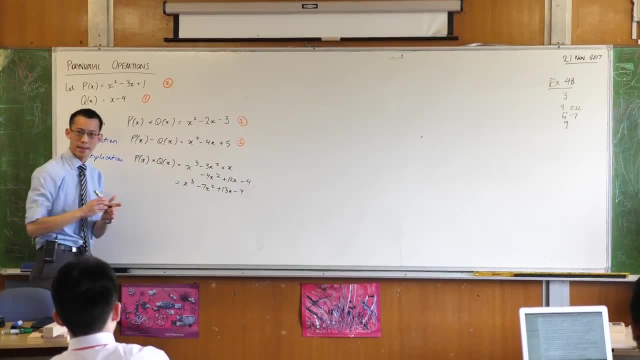 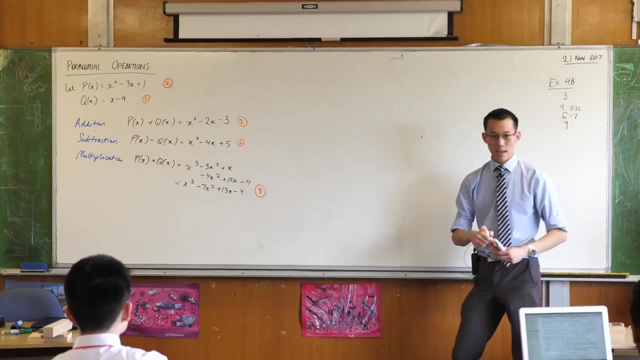 13. And then that constant term is just hanging out there on the end. Okay, So, as we predicted, because we know our index laws, the degree of our product of these two polynomials is the sum of the degrees of the two polynomials we started with. 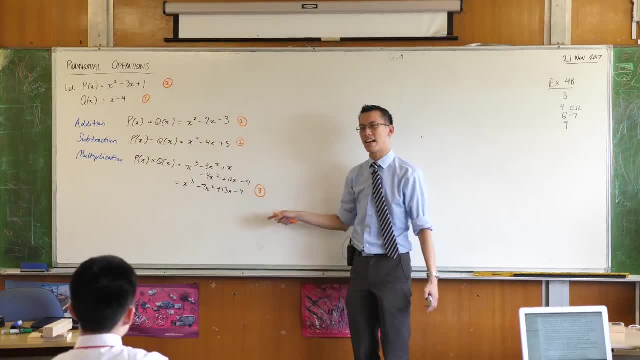 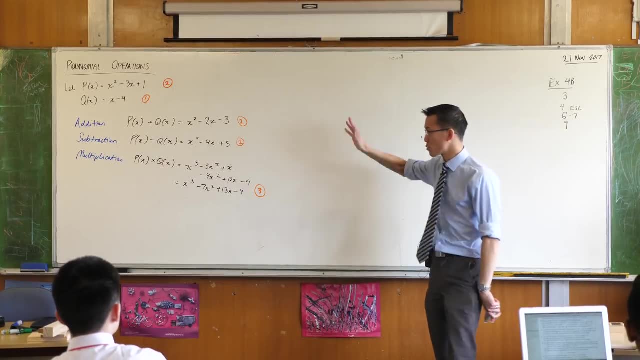 If I had a quadratic and a cubic, you'd expect this thing down here to have a degree of 5.. That would be a quintic. Okay, Not that they come up very often. Okay, Addition, subtraction, multiplication- I've left the last one because it's the harness. 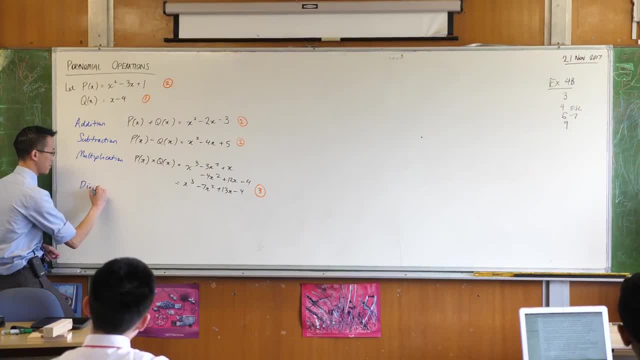 and it's actually what we're going to: devote some energy into Division Okay. Now the tricky thing with this is: if you add two polynomials, you'll get another polynomial. If you subtract two polynomials, you'll get another polynomial. 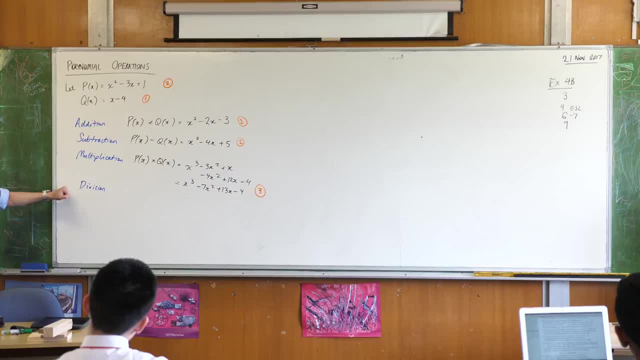 If you multiply two polynomials, you get the idea, But if you divide two polynomials, you may not get a polynomial. Okay, Don't write this down, I just want to give it to you as a point of illustration. If I gave you an easy one like, say this: 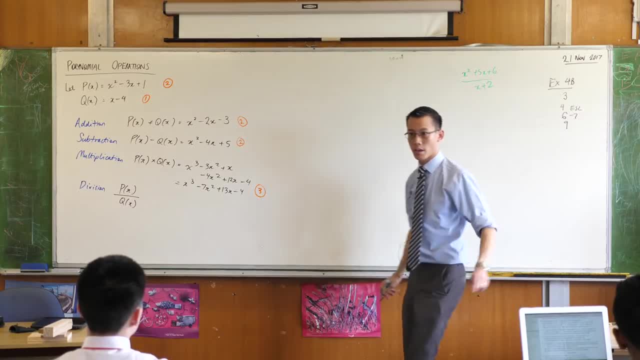 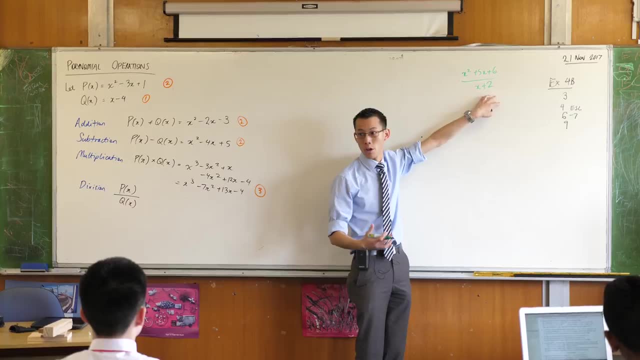 Because you guys know my fondness for this particular polynomial. If I looked at that numerator as a particular polynomial and this numerator, this denominator, as a particular polynomial, you can see here that the answer would be another polynomial. What would it be? It'd be x plus 3.. 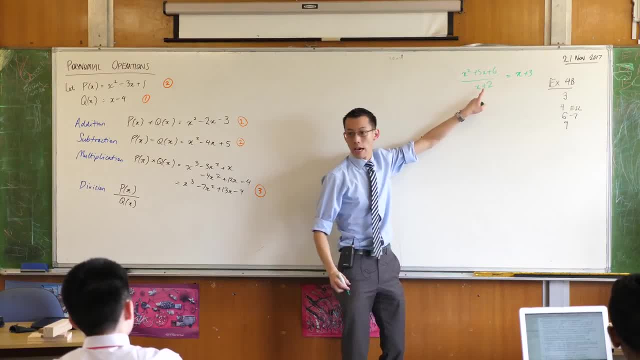 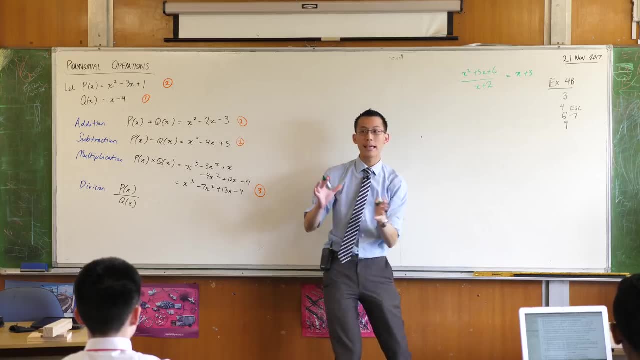 It's worth noting that these two things are not identical because there's a domain restriction on this that doesn't exist over here, but it's still fine Noting that domain restriction. there's nothing wrong with polynomials having domain restrictions. you get another polynomial at the end. 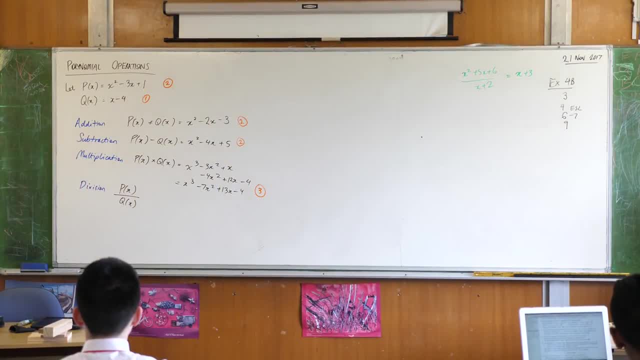 But if you have a look at the p and q that I've given you, you can see that this is not going to fall out nice and neatly, is it? In fact, I've given you one up here which you pretty much Can you even factorise that. 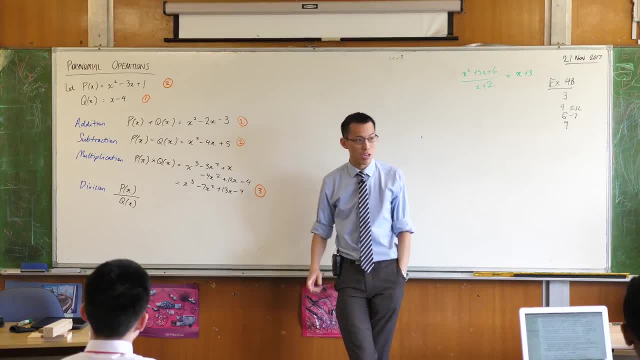 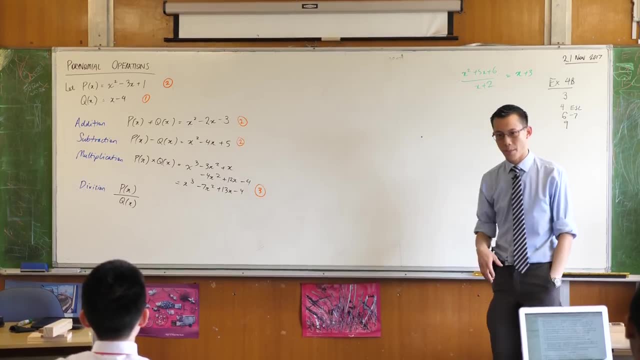 b squared minus 3?? b squared, Yeah, you can use. You're going to have to go to certs, aren't you? But x minus 4 is not going to be one of those factors. So what am I going to do with this? 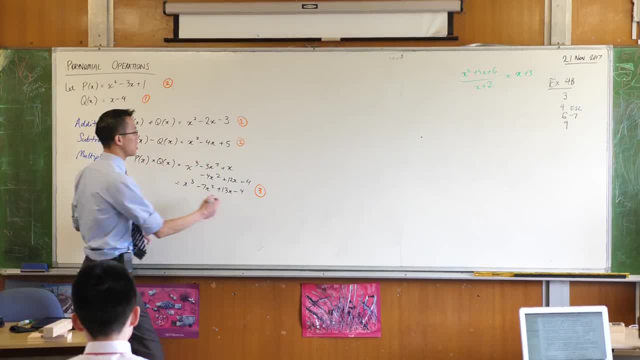 I want you to make a separate subheading because this is such a big deal which is long division. 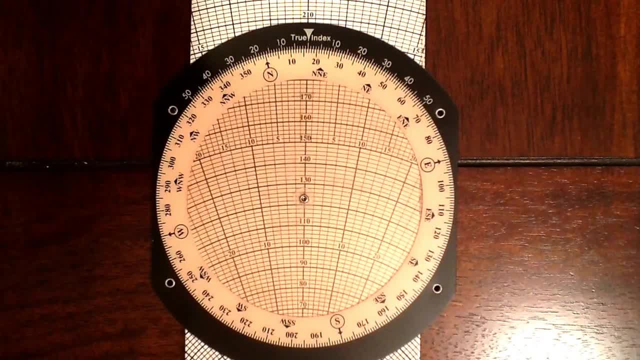 There are two ways to use the wind side of an E6B flight computer. One is: given wind information, you can determine aircraft heading and ground speed. And two: given aircraft heading and ground speed, you can determine wind direction and velocity. The second method, 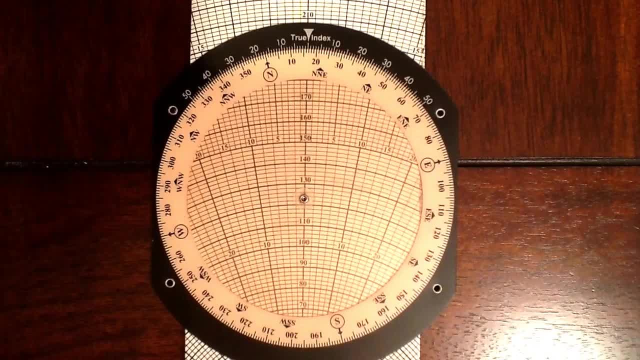 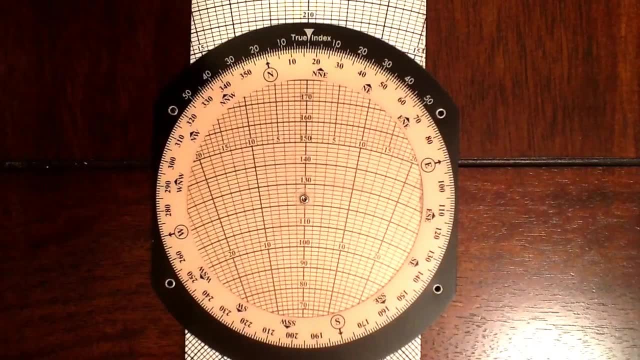 is what we will discuss in this video and it's useful for the instrument pilot knowledge test. Given heading and ground speed, we are going to determine what the wind is doing. In fact, you get a little bit more than heading and ground speed in these problems There.